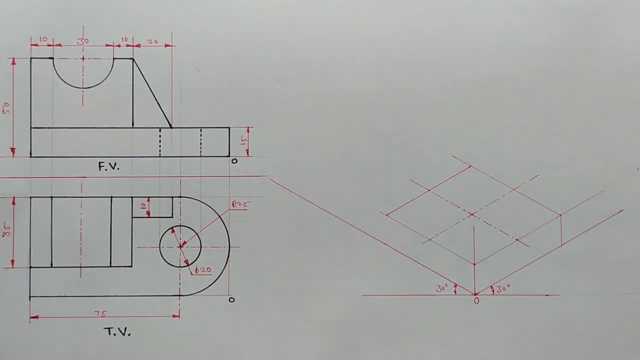 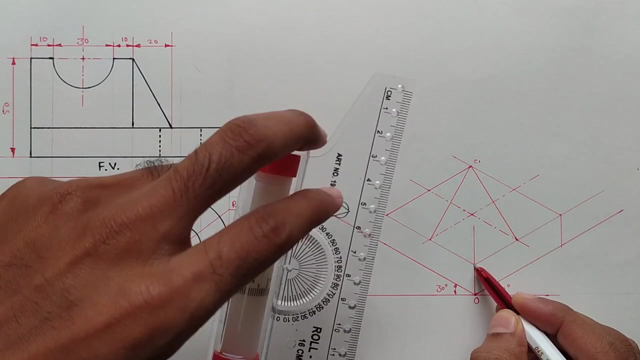 points will be the Main and this points will be the Center point. and that means we have to mark a parallel line from the center line directly улиze at centre field. but be careful because you will draw point two sides simultaneously and mark that point at the centrifugal. 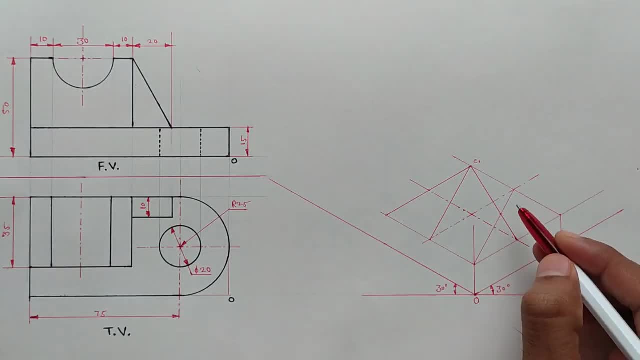 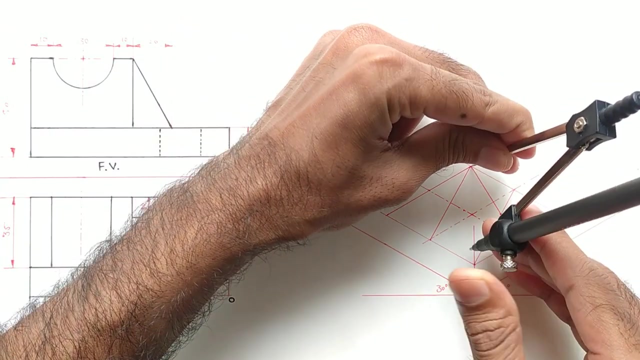 angle near to center point. So let's set this angle And mark point here, coming from the center point, and mark point two sides- This is cm to the edge, and mark points where we are leafing. center point, that is C2. take this distance into compass and draw an arc from these two midpoints, from. 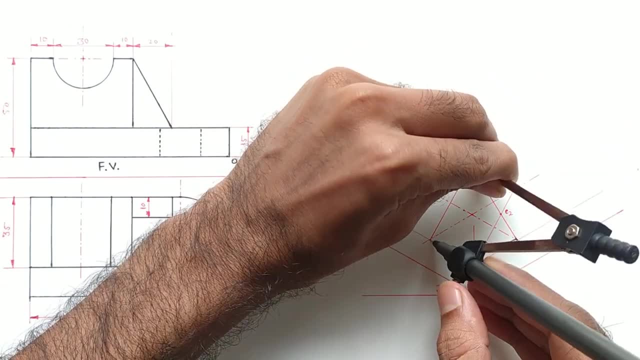 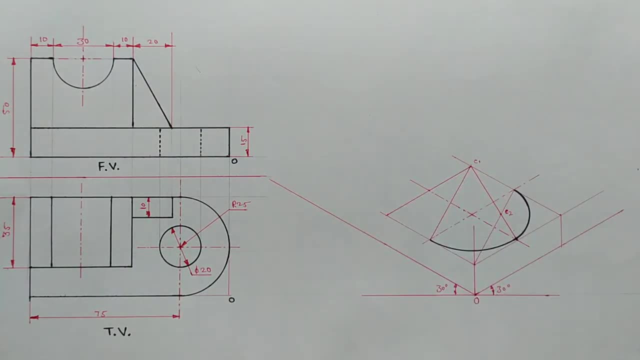 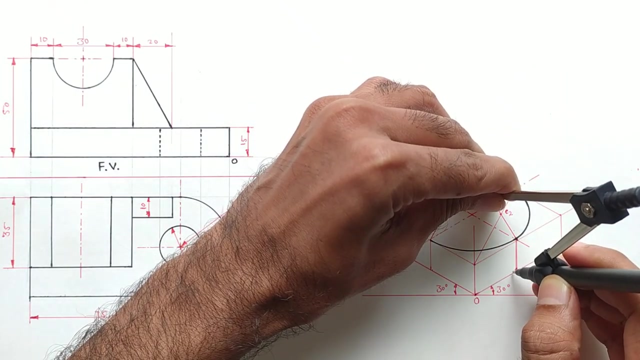 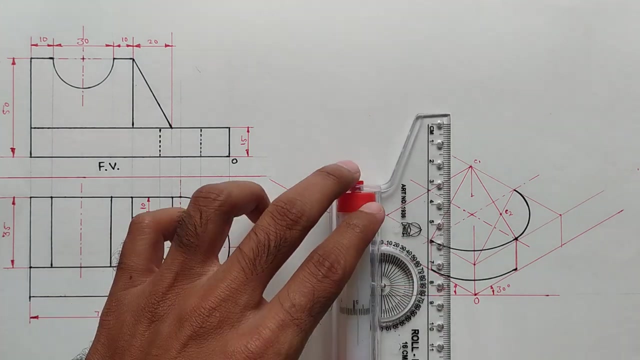 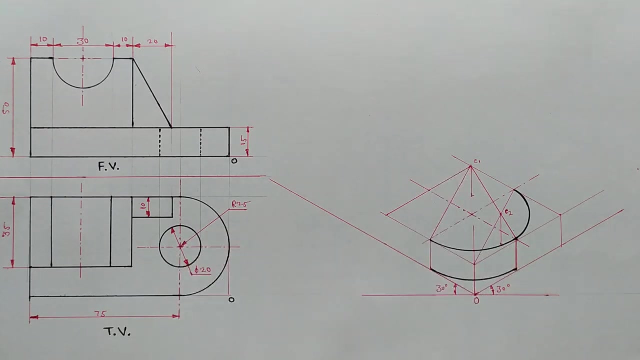 center one. take this distance into compass and draw an arc like this. shift all these points 15 mm below. now again take this distance into compass and with the new center point join these two points. now shift this point also below by 15 mm and with the new center point draw an arc like this and here draw a tangent. 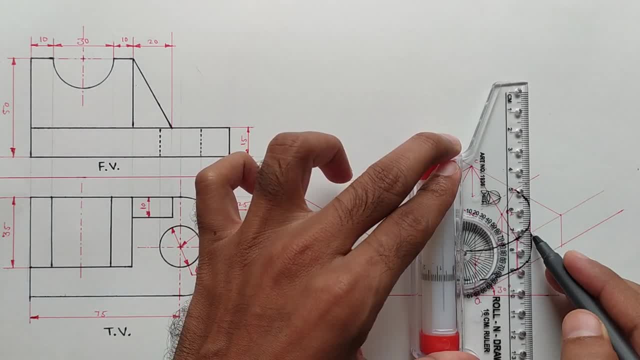 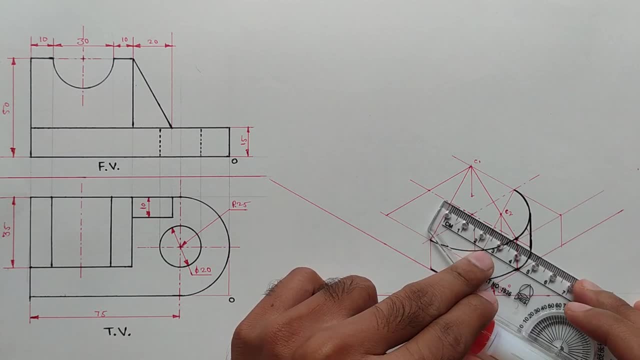 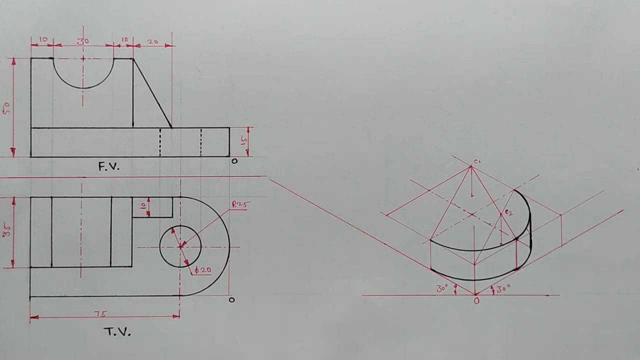 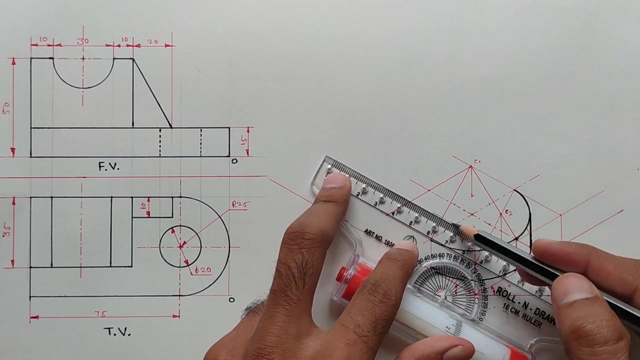 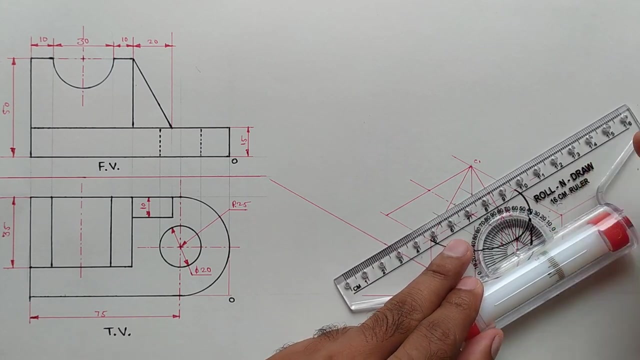 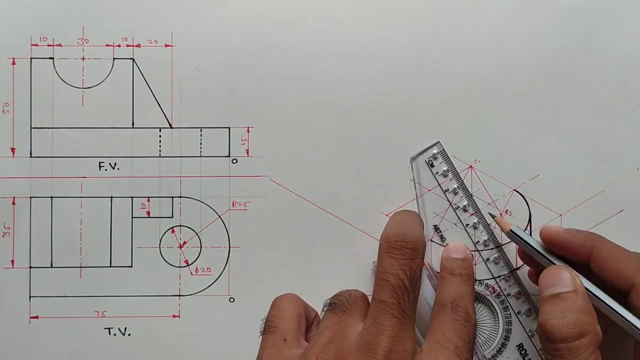 now dark, all feasible portion. ok, now we will construct this circle and to make the circle we should draw an isometric square, and the side of isometric square is 20 millimeters because the diameter of circle is 20 millimeters. here we have drawn the isometric square, Now join the opposite midpoints from 3. 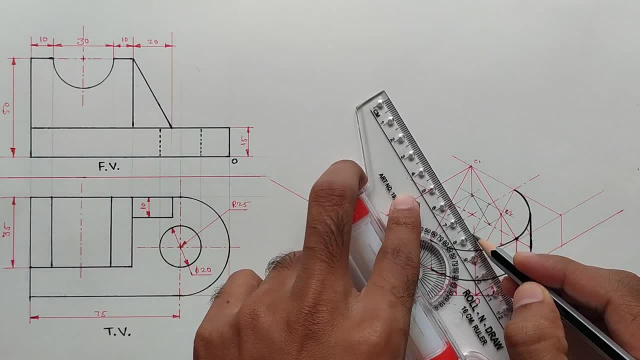 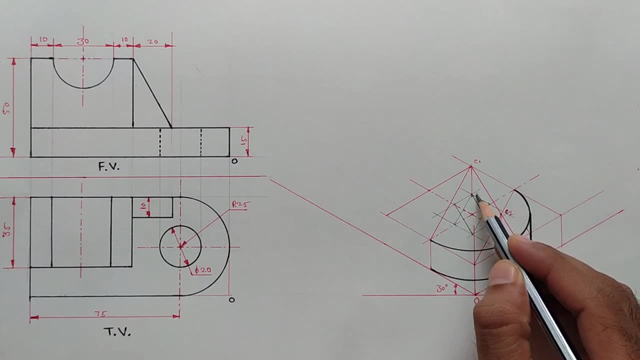 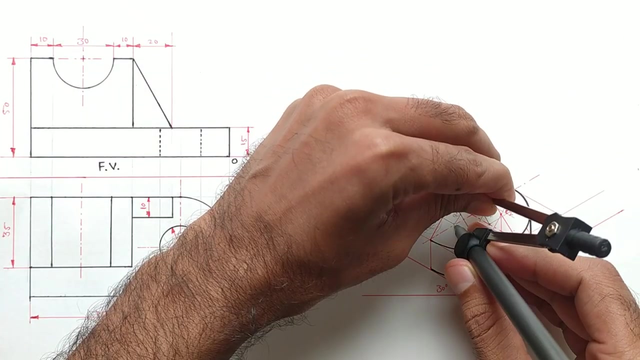 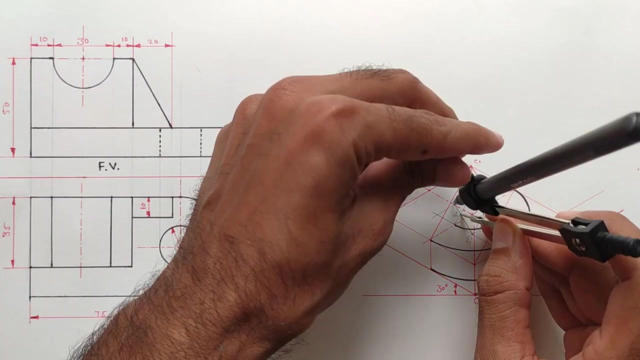 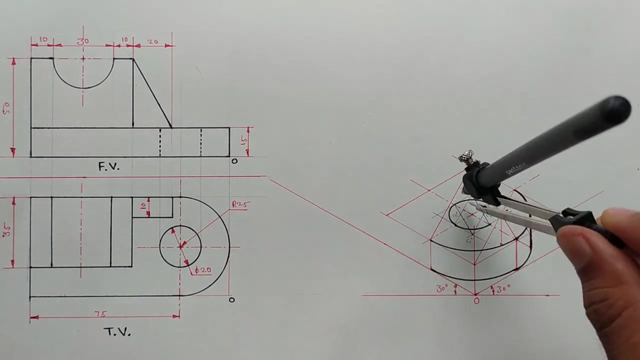 angles like this. now, these are the center points. all these are the center points. now take this distance into compass and draw an arc from these two midpoints, and do the same from the opposite center point. take this distance into compass and draw an arc from these two midpoints and do the same procedure for. 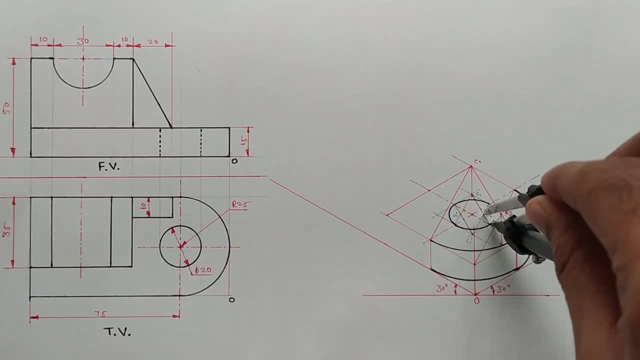 this side also shift this center point below by 15 millimeters, because the height of this block is 15 millimeters. take this distance distance into compass and with the shifted center point just check whether it is visible or not. now, here the circle is not visible. 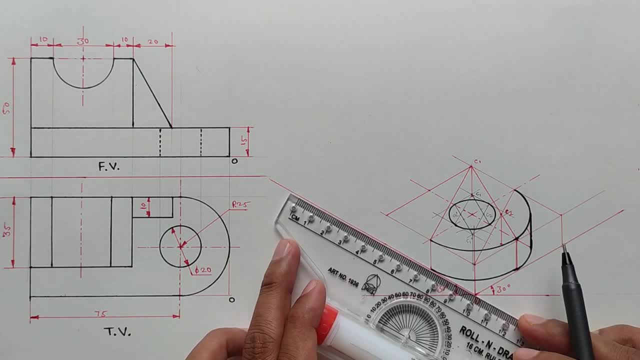 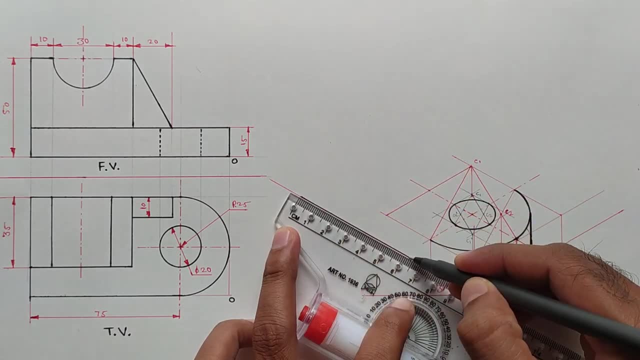 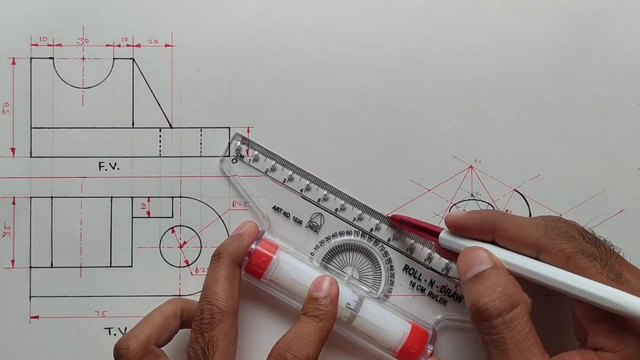 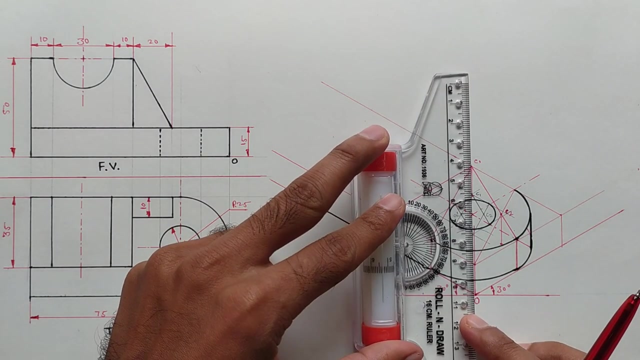 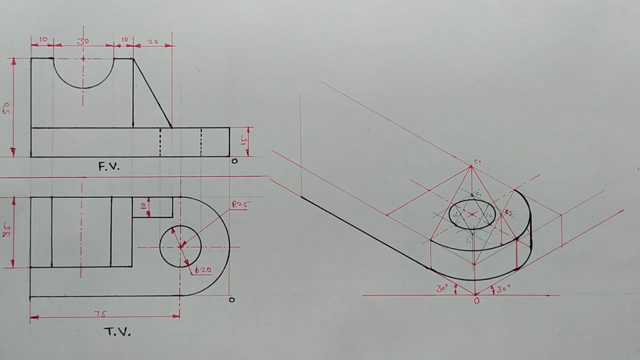 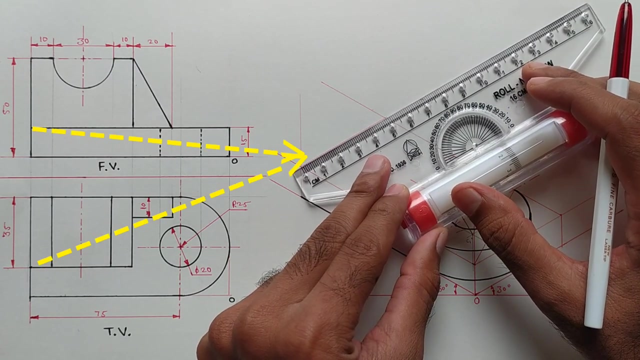 now dark on this line and this distance is total 75 millimeters. you now- I am shifting all these points back- and draw a vertical line from this point, a set scale parallel to x-axis, and draw a line from this point- point on 15 millimeters here- and draw parallel line to the y axis from this. 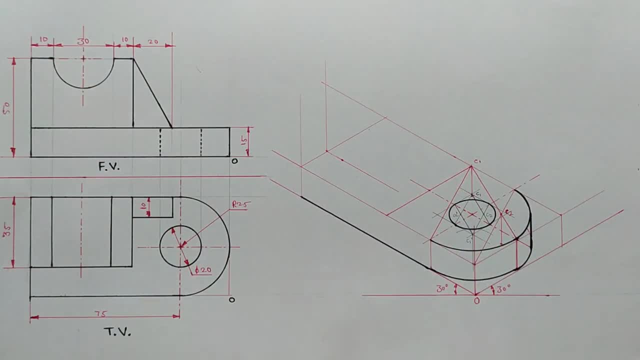 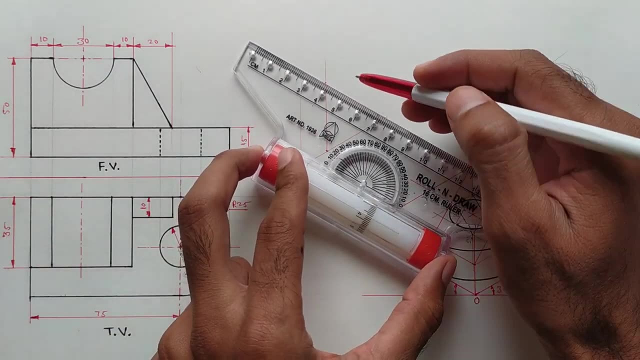 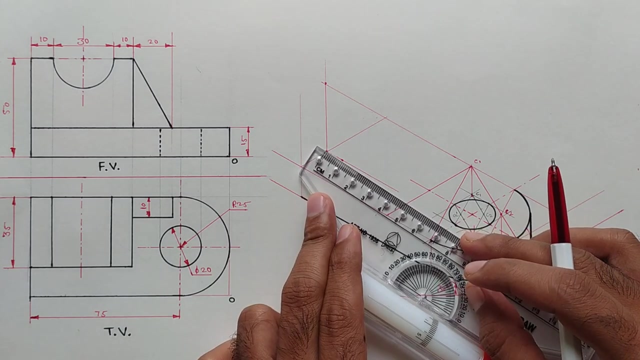 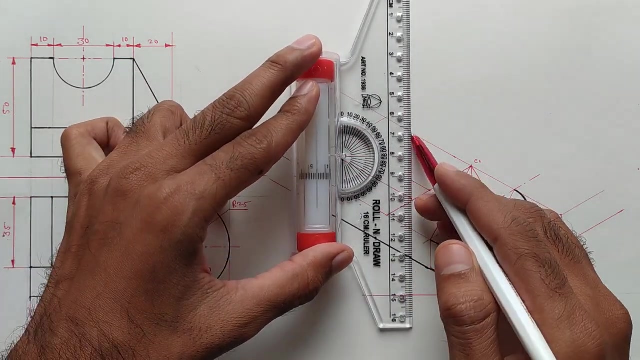 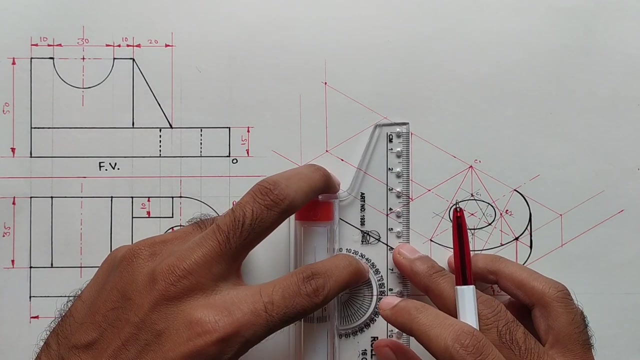 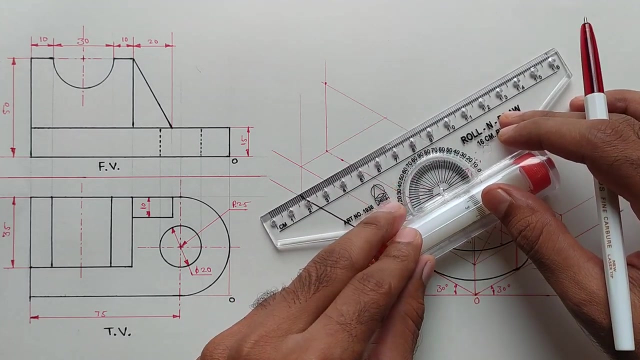 point and also draw a vertical line from this point and Mark 35 distance. here mark point on 15 millimeters, mark point on 15 mm and draw vertical line from this point, and here the distance is also 35 mm. Now set scale parallel to the x axis and draw the lines from these two points. 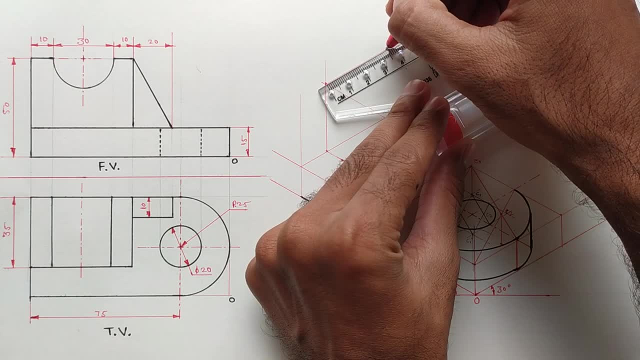 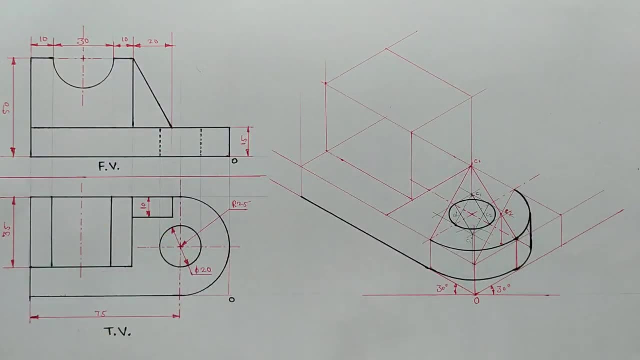 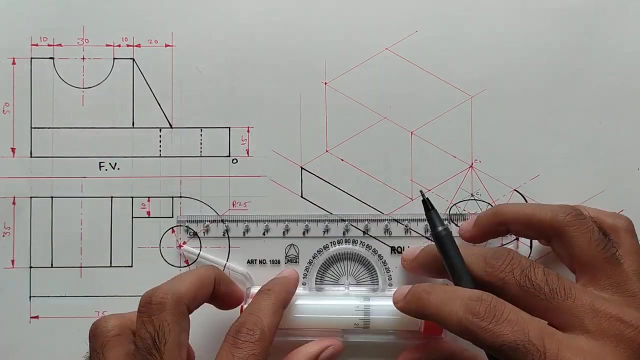 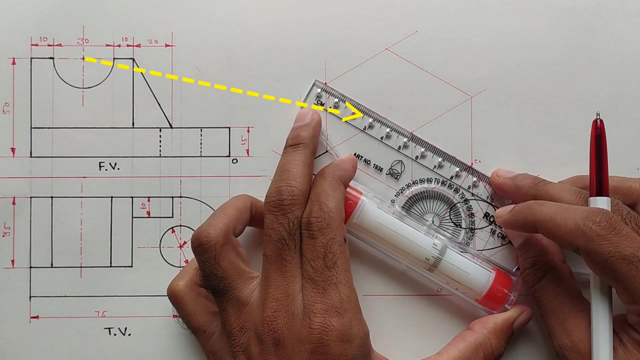 Now, here measure 35 mm distance and mark the point and draw the parallel line like this, and here draw the vertical line also Dark this line and this line also, and this line should be dark. Mark midpoint on this line. here We have to draw the semicircle. 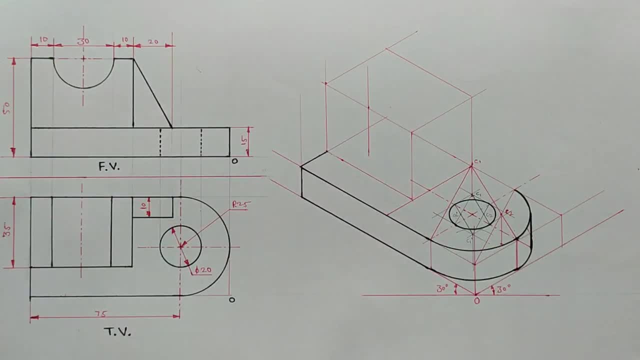 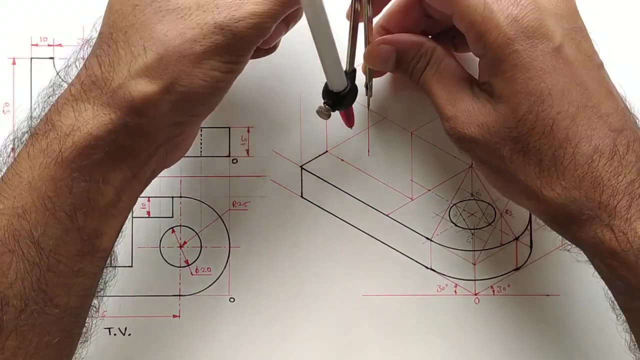 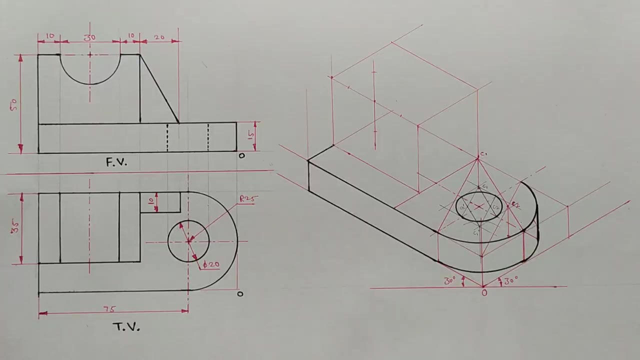 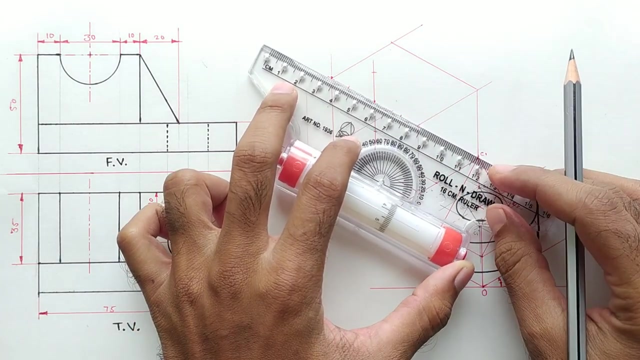 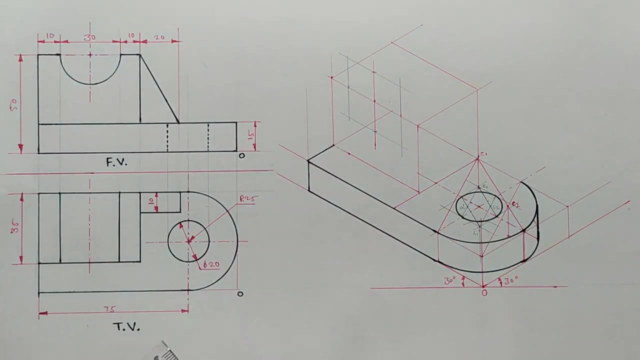 The semicircle which is appearing in front view. Again, here we have to make an isometric square. Ok, the isometric square is completed. Now join the opposite midpoints from the big angle. This is center 1 and this is center 2.. 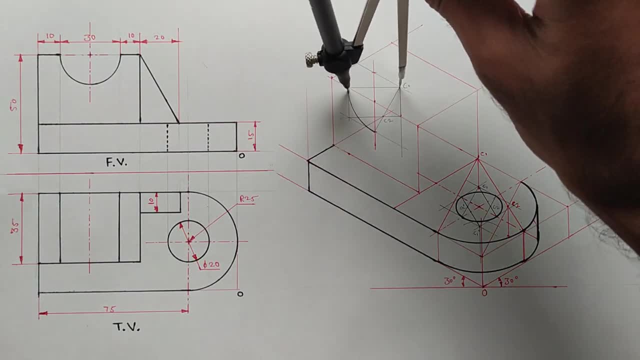 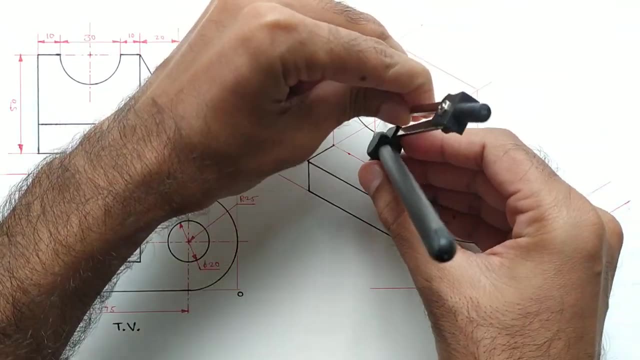 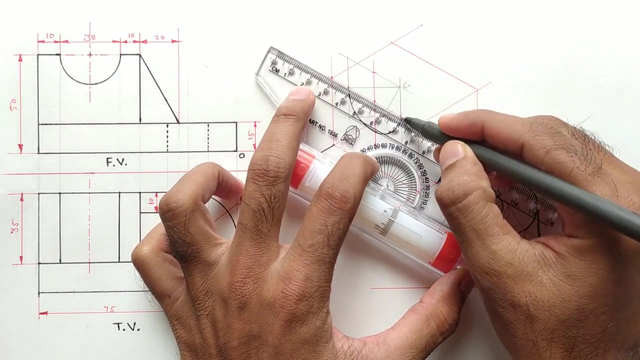 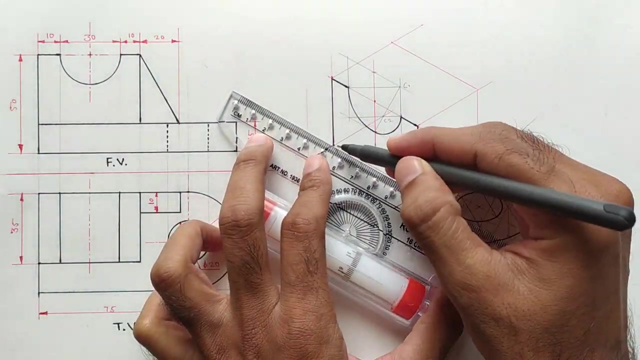 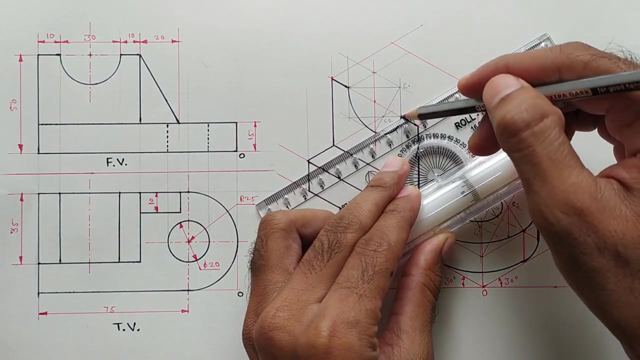 Now take this distance into compass and, with the center 1, draw an arc like this and draw the arc from center 2.. The center 2 also like this. Here the semicircle is completed. Now dark, all the visible edges. Now draw a line from this point and this point also, and draw the lines from the center points. 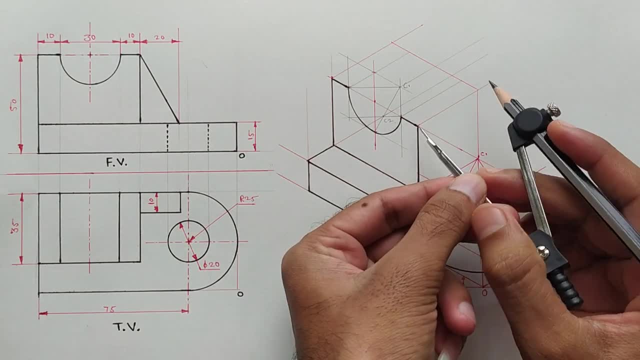 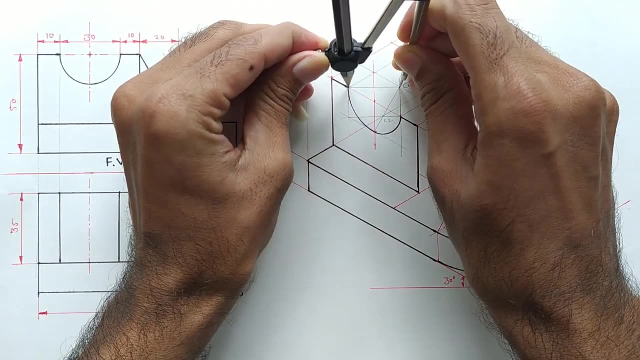 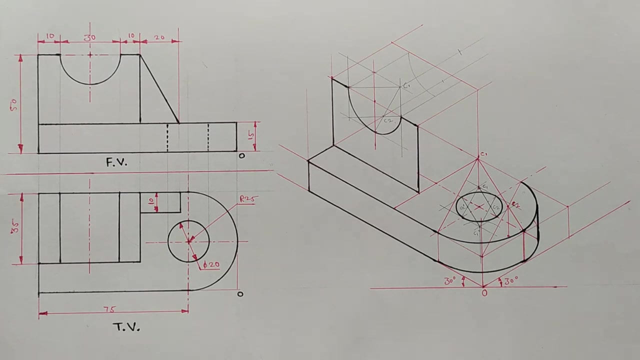 also Mark 35 mm distance. Now draw a line from this point and this point also, and draw the lines from the center points also Mark 35 mm distance on the lines which are drawn from the center points. Take this distance into compass and with the new center point draw an arc like this: 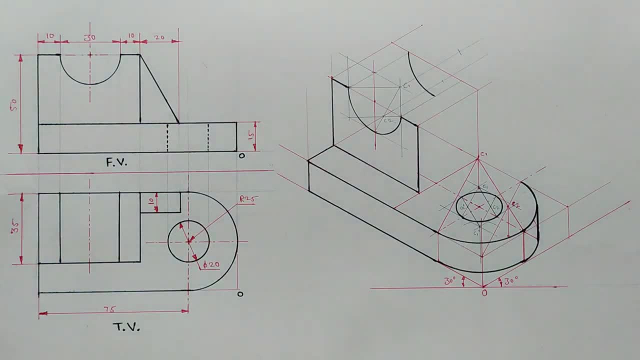 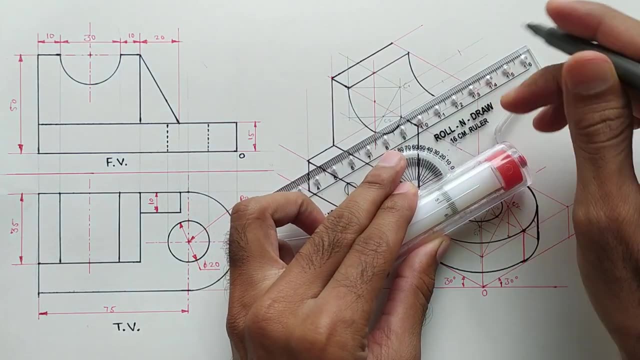 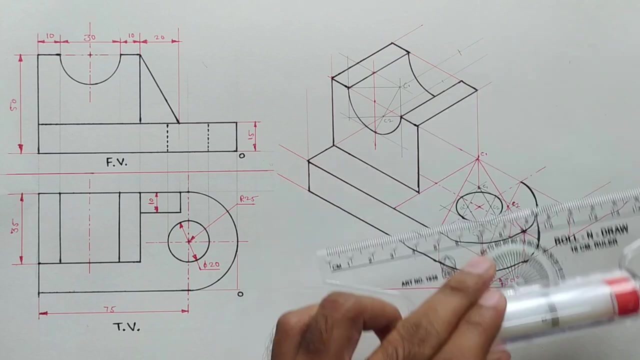 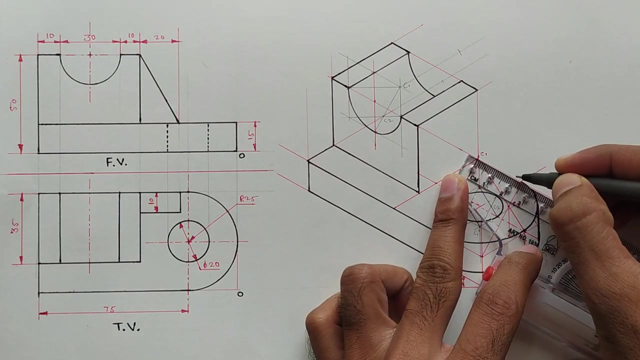 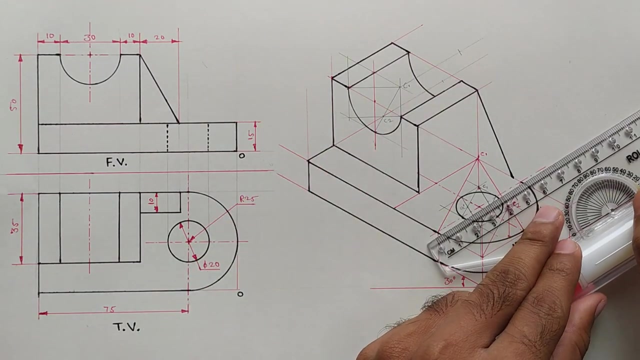 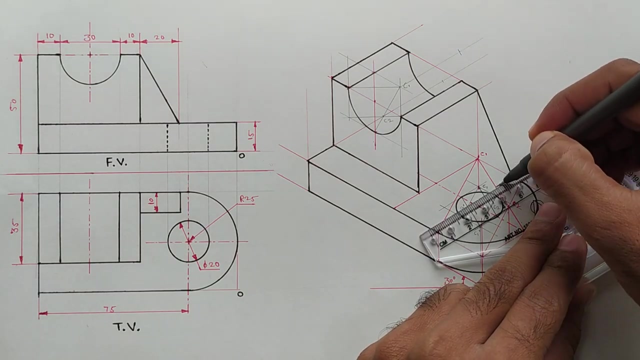 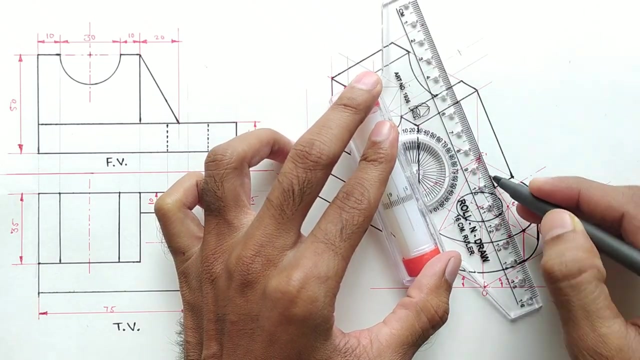 And dark the visible portion Now, dark all these edges. Now we will draw this rib and here this distance is 20 mm. So mark point on this line and join these two points. The width of the rib is 10 mm. So draw a line and draw parallel line like this: 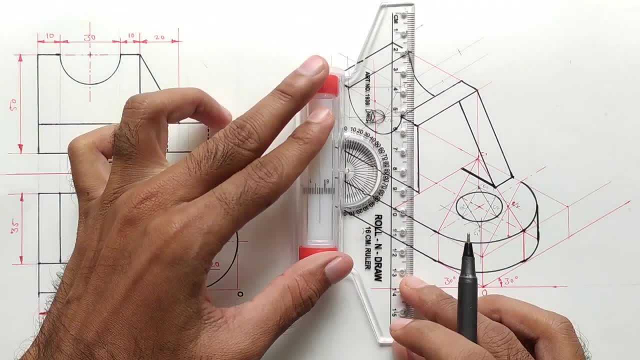 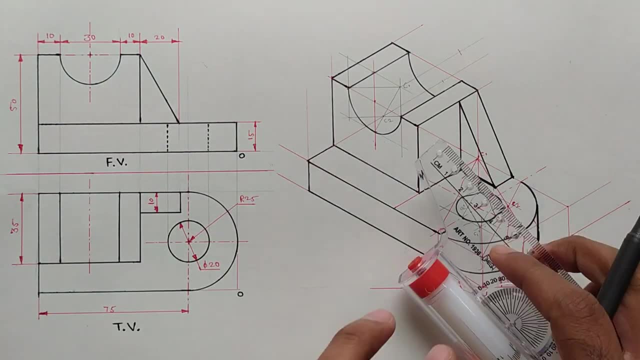 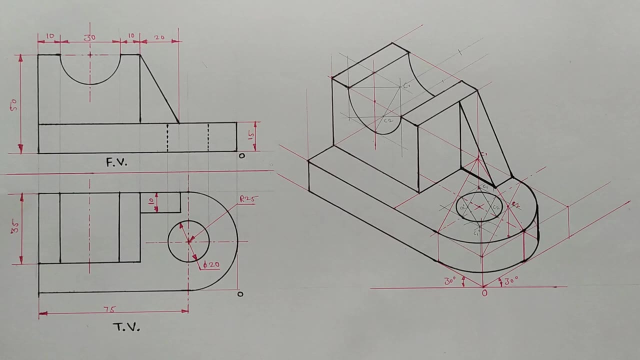 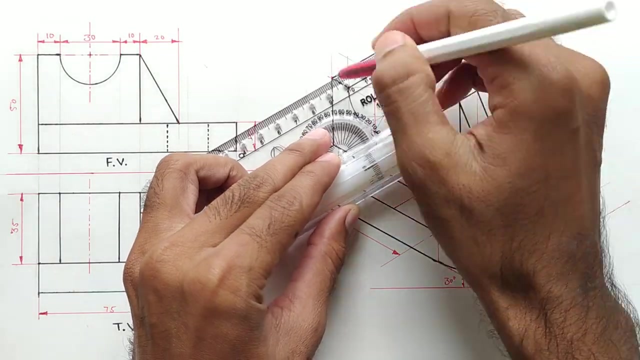 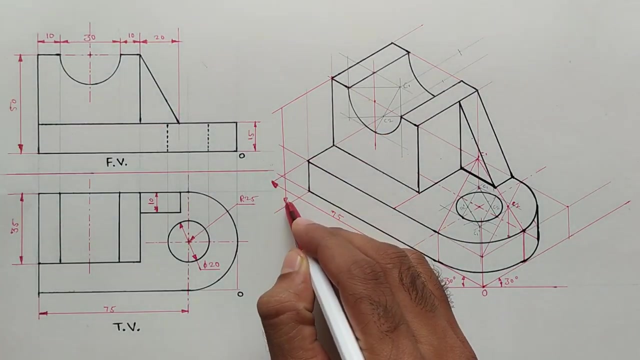 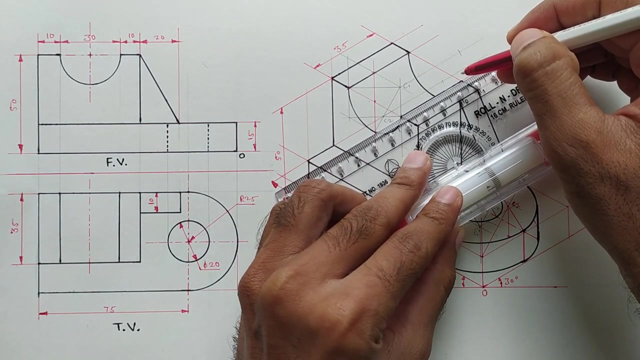 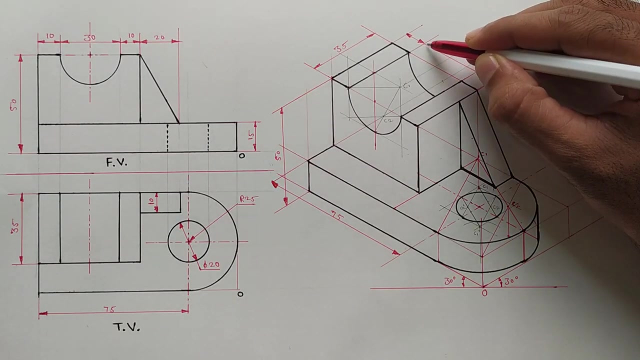 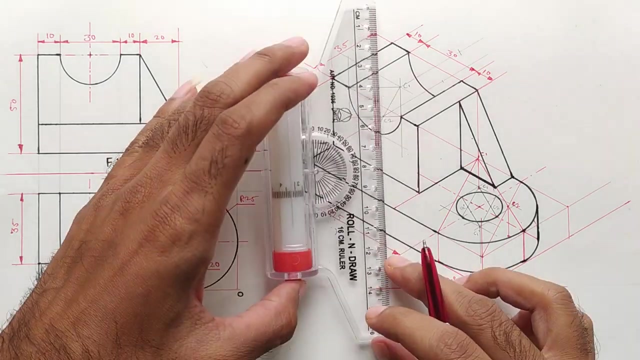 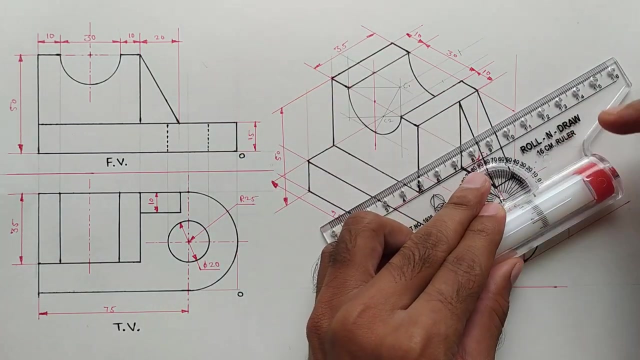 Now draw the line here and draw vertical line here like this and make this line dark. Draw this small line also Now. here the object is completed. Now we should give all the dimensions which are appearing in front view and the top view, If you have plastic cutting. 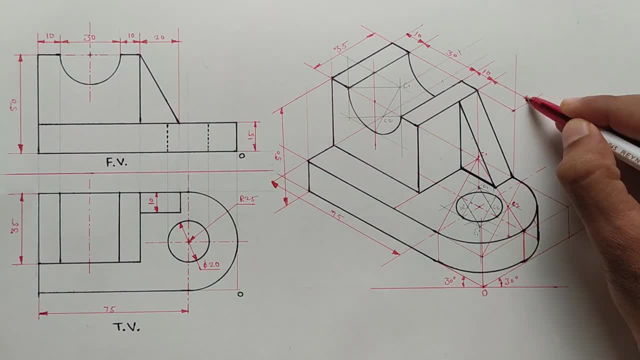 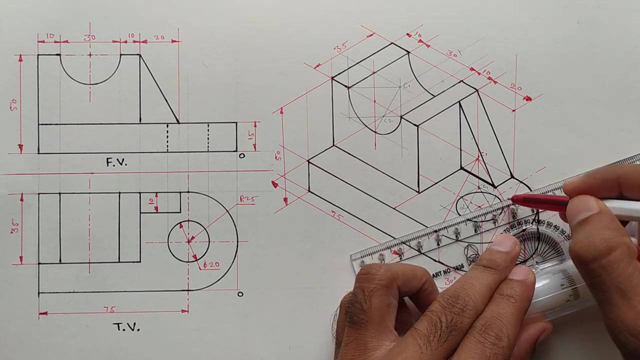 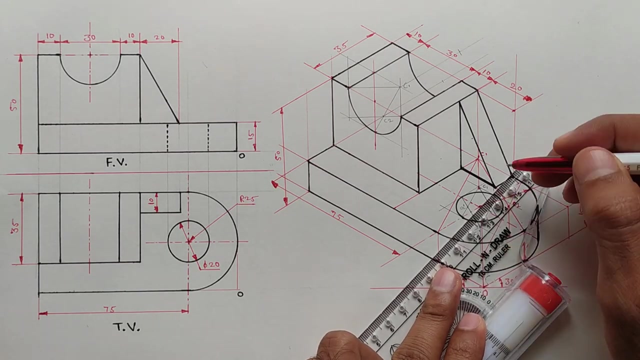 and pipe and buildwork rules in your design, if you want to. there is dancer's knives. Here is the painting, Here is the wisdom. you, you.